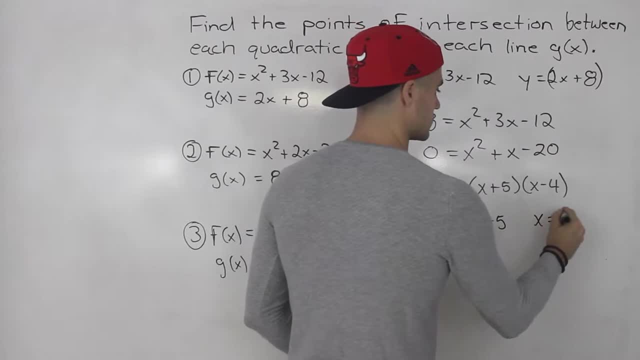 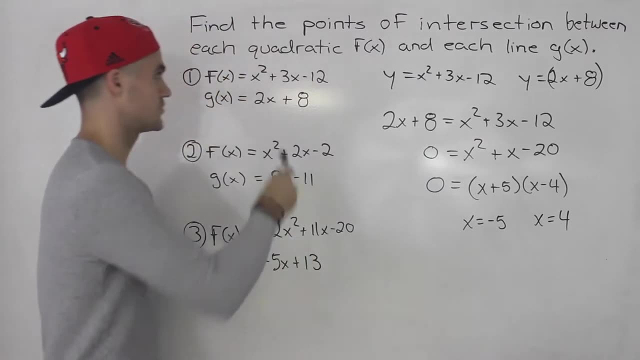 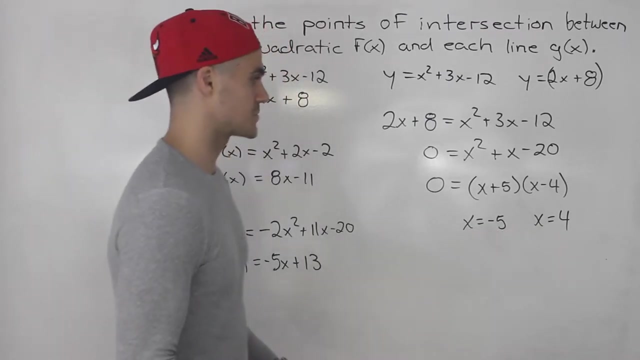 tell x is negative 5 or x is equal to 4. so, because we got two solutions, there's actually two points of intersection between this quadratic and this line. so we have the x values at which that happens. what are the corresponding y values? well, starting with this, negative 5. 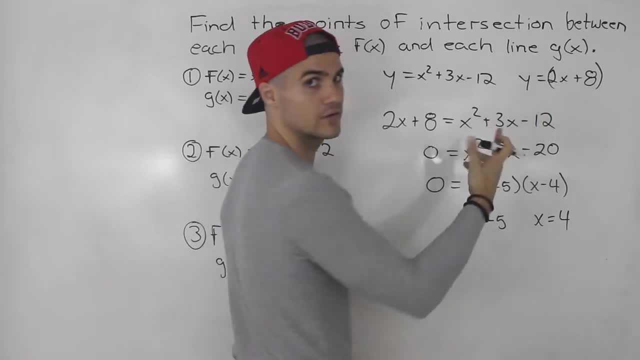 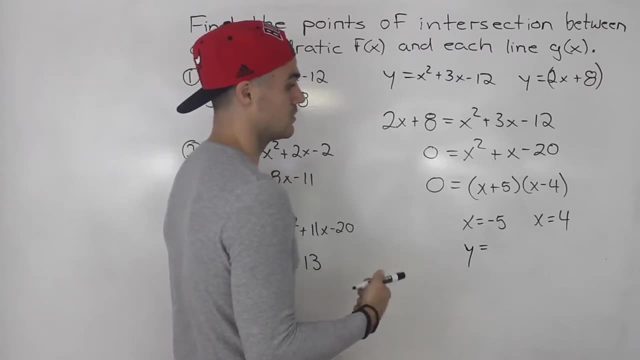 you could take this negative 5, plug it in here or plug it in there. you'll get the same y value, or you should get the same y value. that's actually a good way to check. if you do get the same y value, then you know this is correct. so, plugging in negative 5, i'm going. 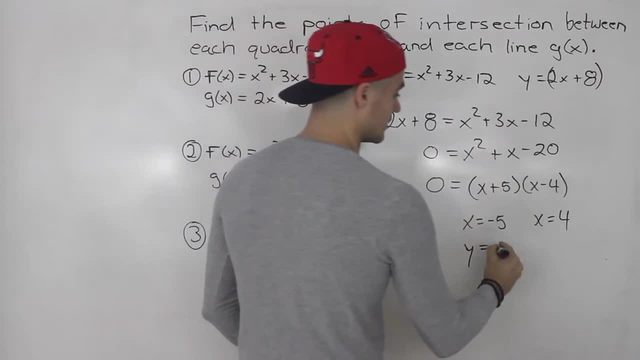 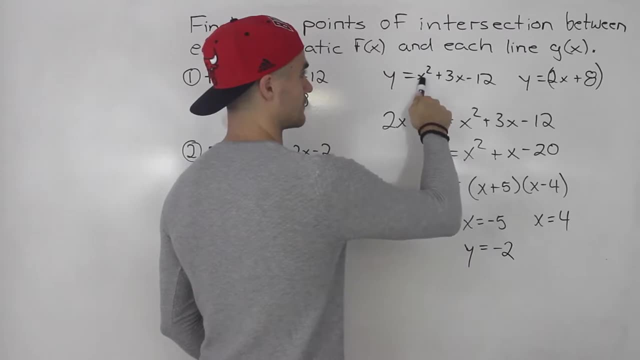 to plug it in here, 2 times: negative 5 is negative. 10 plus 8 gives us negative 2. if i take negative 5, plug it in here, i'd have uh negative 5 squared, which is 25. uh minus 15, which is 10, 10 minus. 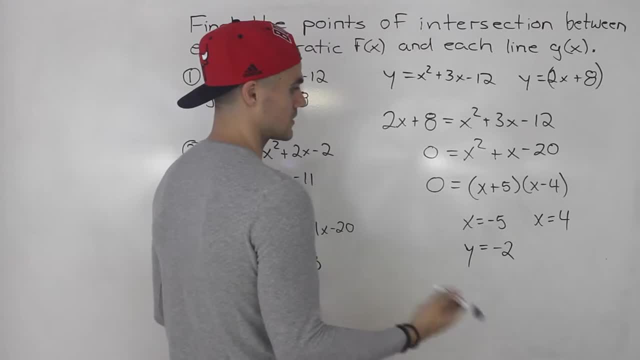 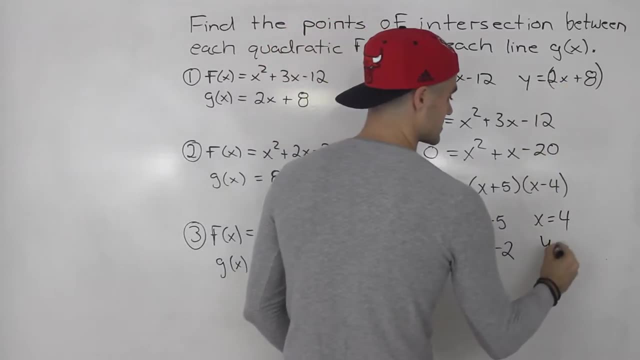 12 is negative. 2 as well, all right, so i get the same y value in both if i plug in 4. i plug in 4 here 2 times. 4 is 8 plus 8 gives us 16, and then if i plug in 4 here, i'll have: 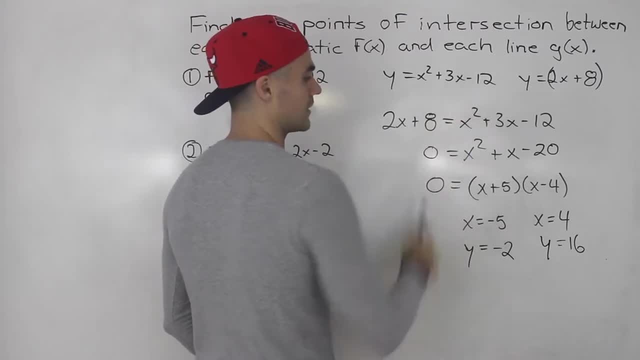 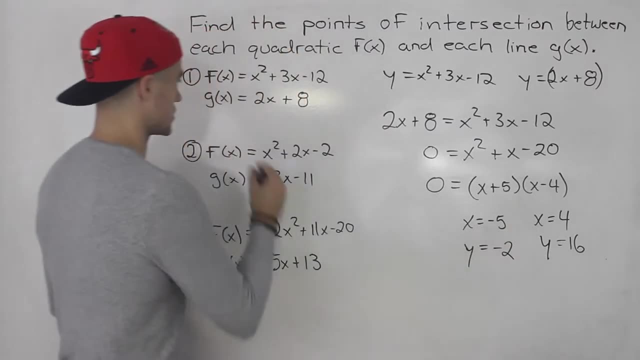 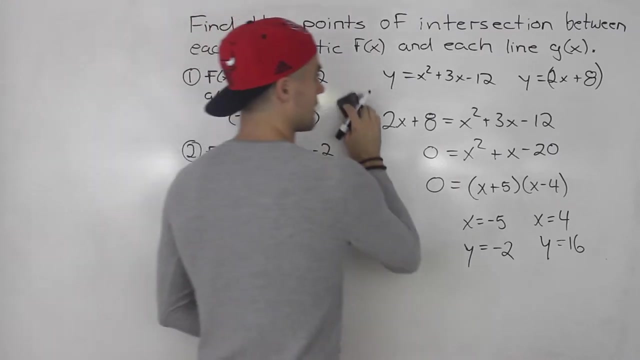 uh, 16 plus 12, which is 28, 28 minus 12 gives us 16.. right, so those are the two points of intersection here. so we have negative 5 and negative 2, and then we have four and 16, like that. so the way that this looks um visually. 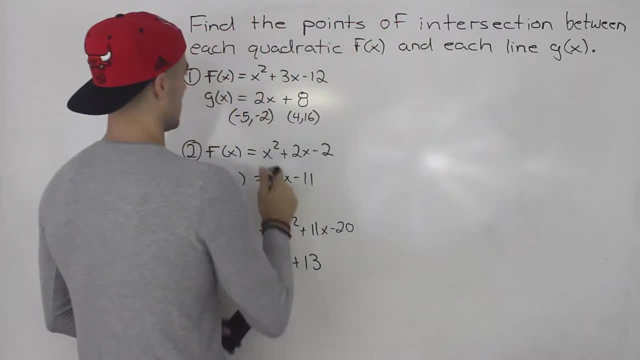 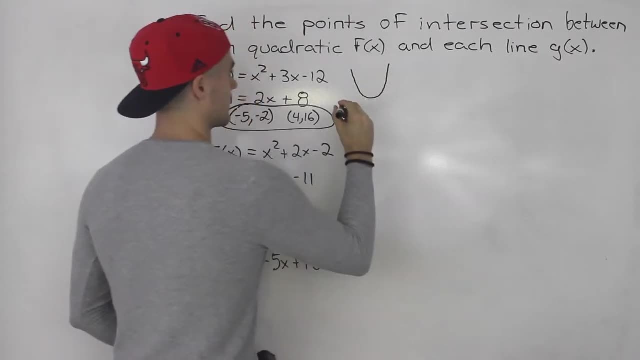 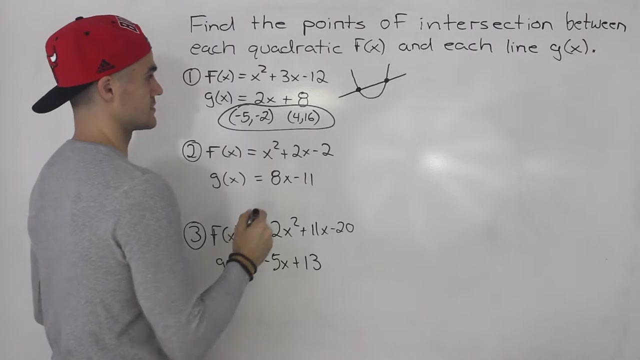 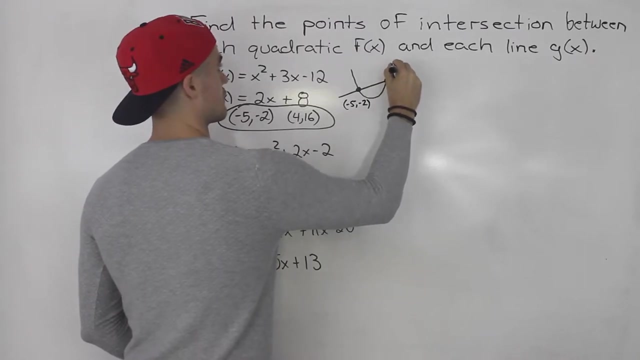 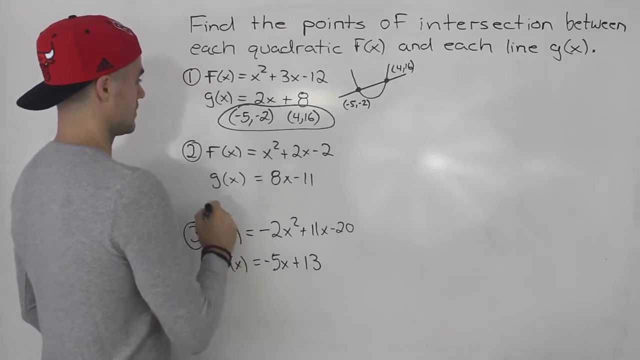 is uh. let me just circle this here is: we have a parabola and then we have a line that is going through it and it's intersecting at two points. so these two points: uh, negative 5, negative 2. this point here is uh, 4 and 16.. okay, moving on to number two, we got f of x equals x squared plus. 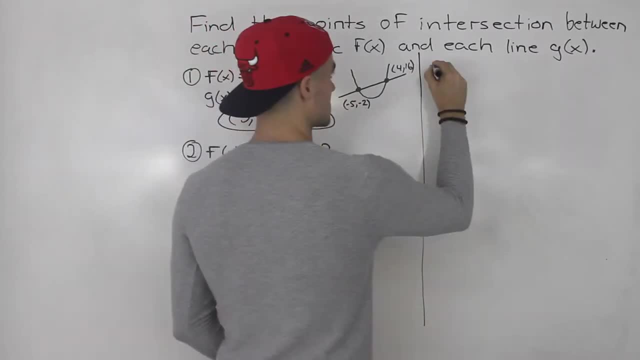 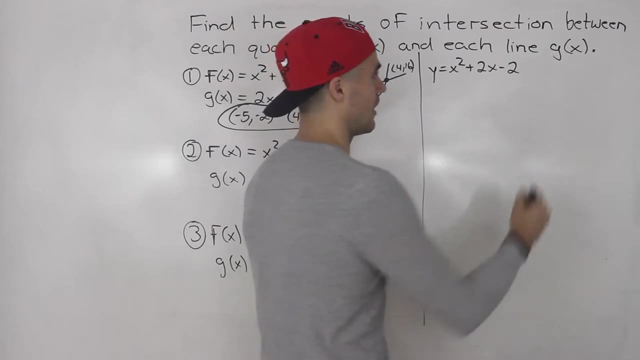 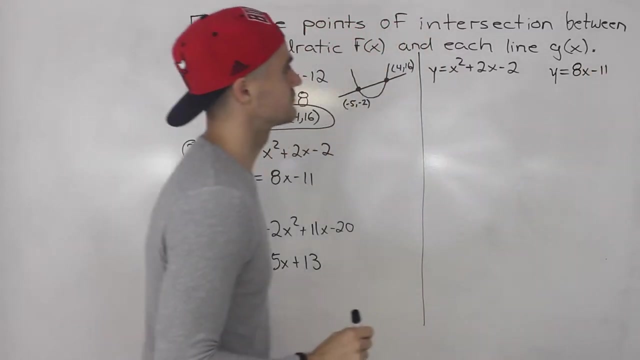 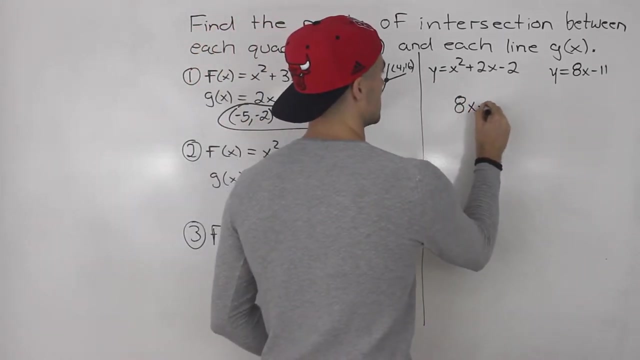 2x minus 2. so let me split this up here. so we got y equals x squared plus 2x minus 2, and then we have the line y equals 8x minus 11.. so same thing, just make the y values equal. so we'll have 8x minus 11 equals x squared plus 2x. 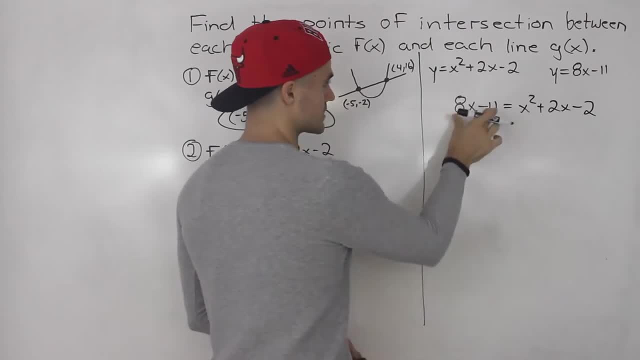 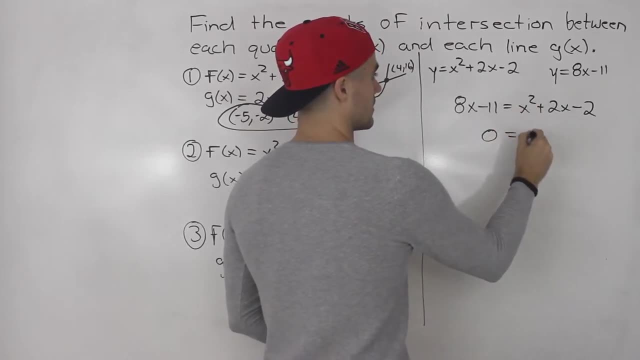 minus 2.. i want to bring everything over to one side. let's bring all of this over to the right side, so we'll have 0 left on the left side. x squared stays 2x minus 8x gives us negative 6x. 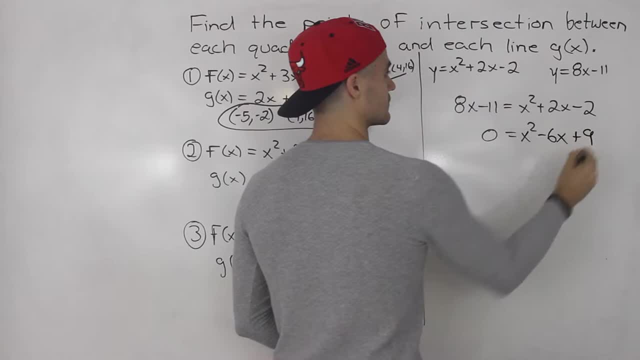 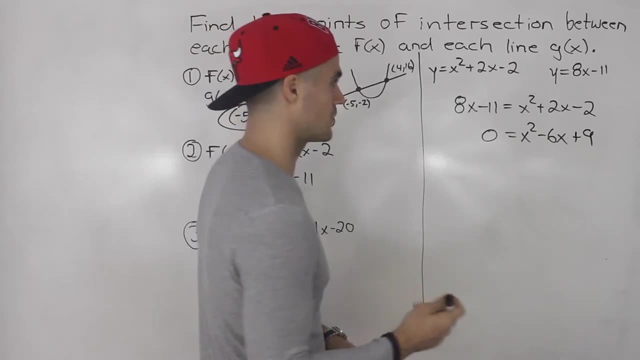 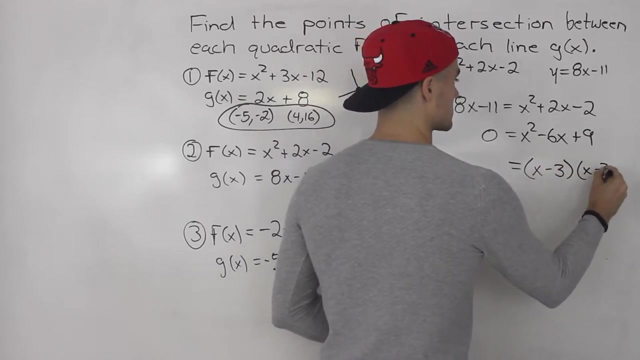 then negative 2 plus 11 gives us positive 9.. then from here, this is just a quadratic equation factor. it, or throw it in the quadratic formula. this actually factors smoothly into x minus 3 times x minus 3. it's a perfect square trinomial. 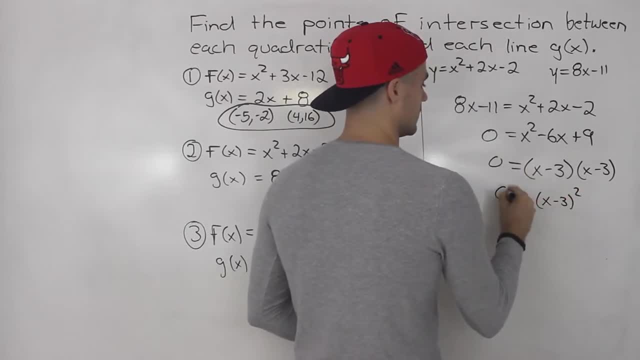 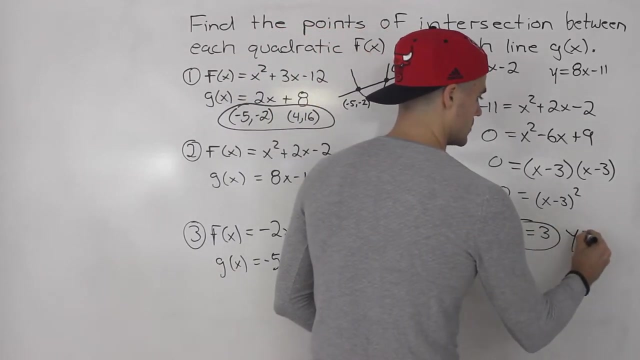 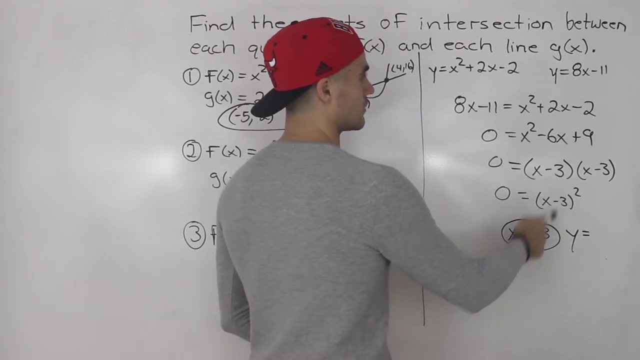 so x minus 3 squared. so here there's only one solution, an x value of 3, so there's only one point of intersection in this case. and then if you want to get the corresponding y value, plug in 3 into either the quadratic or the line should get the same y value. so plugging in 3 here 8 times 3, 24 minus 11, gives us 13. 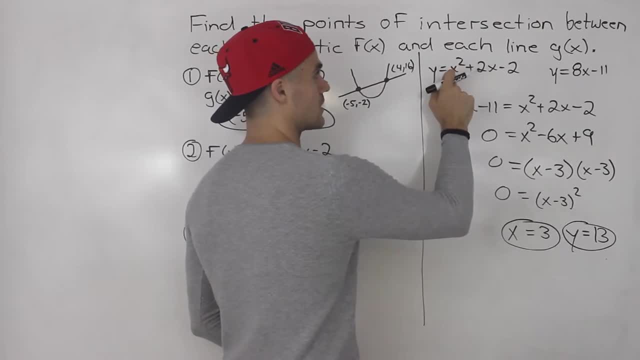 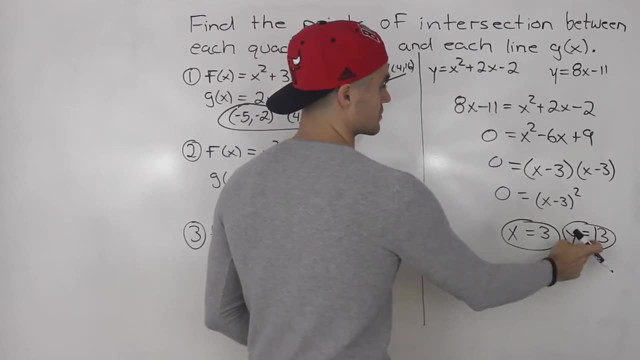 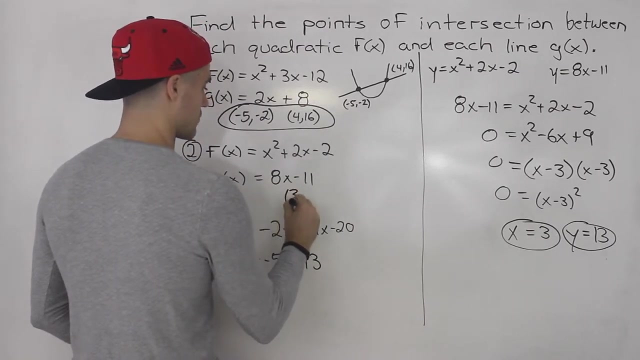 plugging in 3 here: 3 squared is 9 plus 2 times 3 is 15 minus 2 gives us 13 as well. so solution for this one is there's only one point of intersection and it's at 3 and 13.. so the way this looks visually is: you maybe have 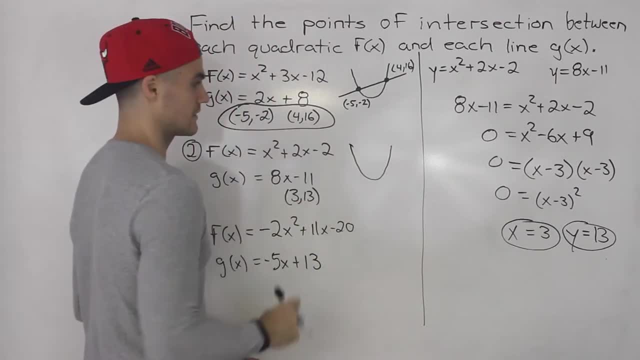 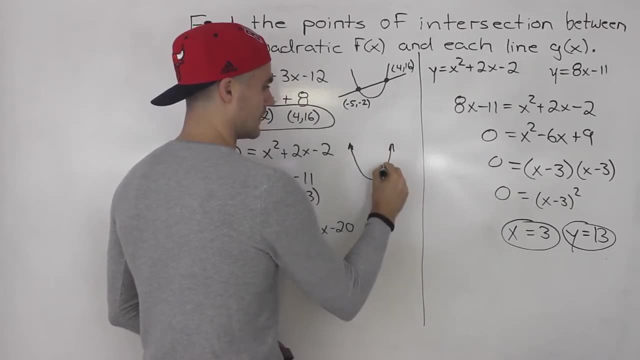 a quadratic like this. by the way, this is not perhaps exactly how it's going to look, but it's going to look something like this. so you have this quadratic here, and then there's only one point at which the line and the quadratic intersect, so this is 3 and 13.. 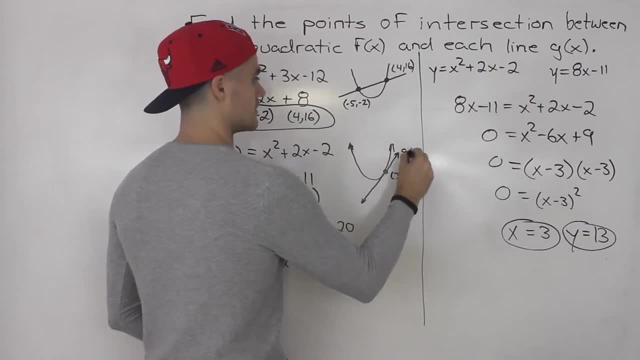 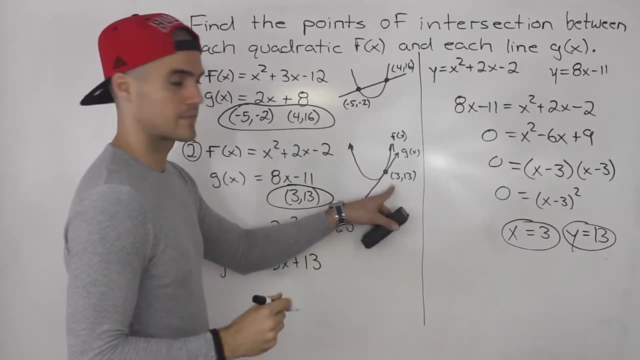 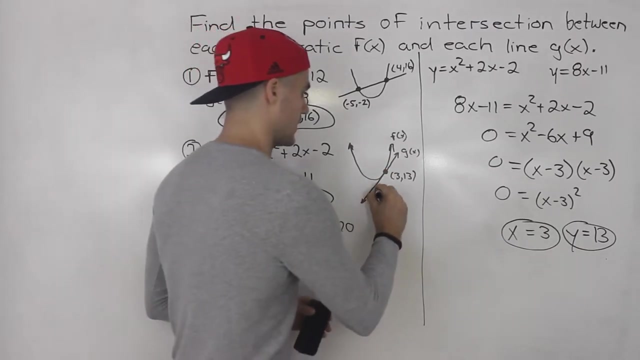 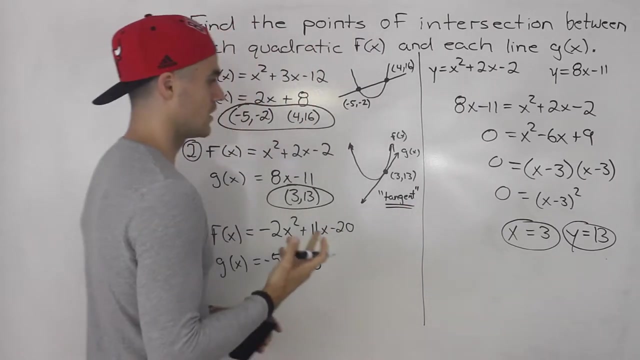 so this line here g of x and this quadratic here is f of x. Another way to describe this here is that the line is tangent to the quadratic. So whenever you see the word tangent come up in this section, what they're pretty much saying is that the 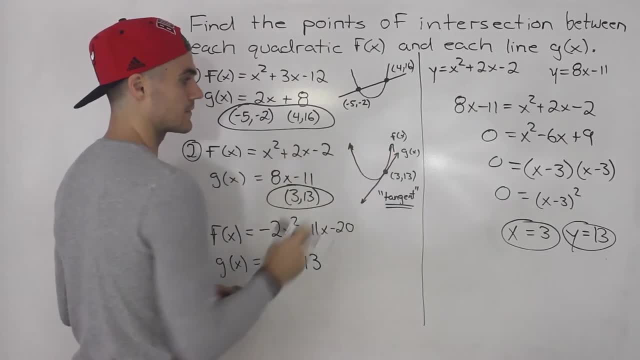 line and the quadratic have one point of intersection. when you see the word tangent come up- And we're gonna be actually doing problems in future videos where I bring this word up and just how to deal with it- You'll probably see it in your textbook. Whenever you see tangent, the line and the quadratic have one. 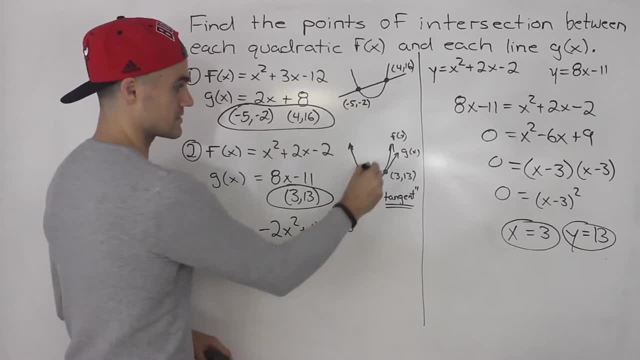 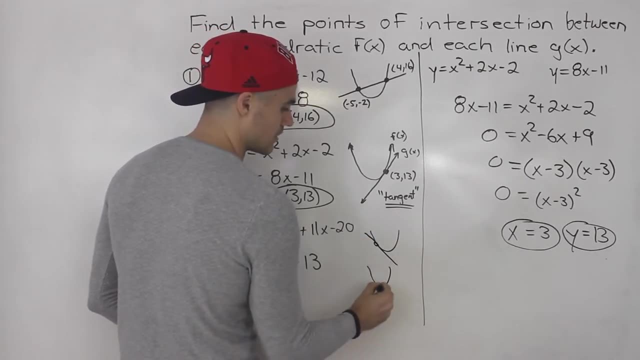 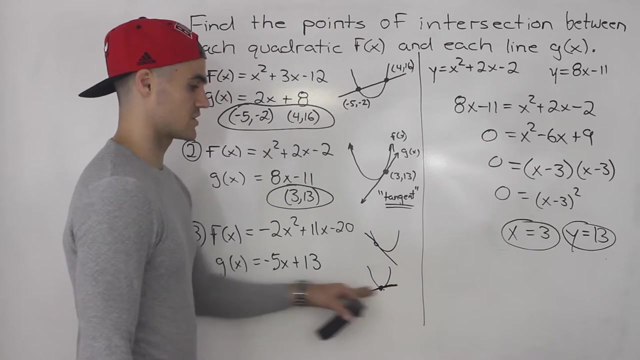 point of intersection. That's what it means. So this is how it looks visually, And then it could also be like a downward sloping line, like that, Or it could even be on the, on the vertex, So it could be a horizontal line. Slope would be zero in that case, But in this case we know the. 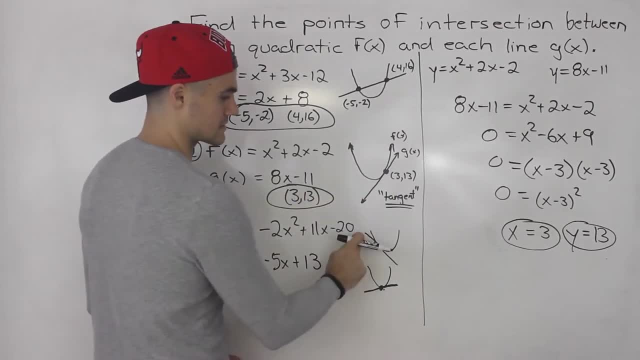 slope is positive. so we know it's gonna look something like that. This is a negative sloping line and then this line has a slope of zero. But either way, all cases- they are tangent. The lines are tangent to the quadratic. There is one. 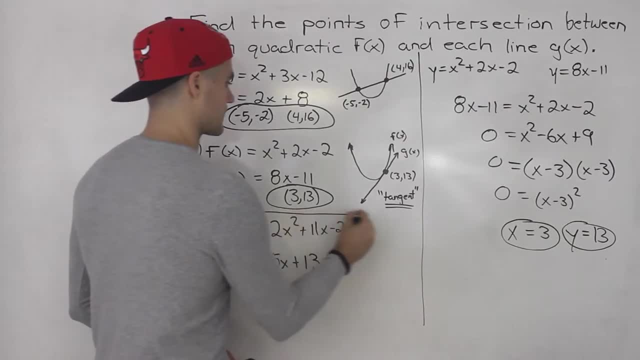 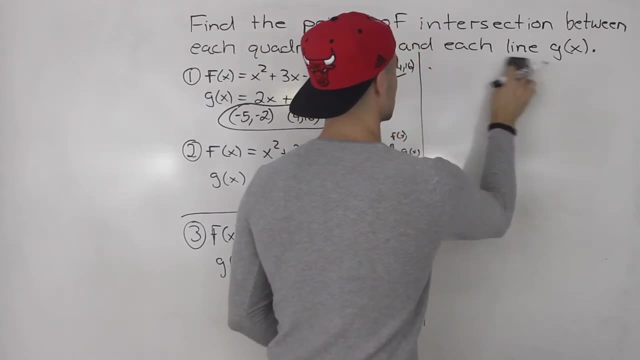 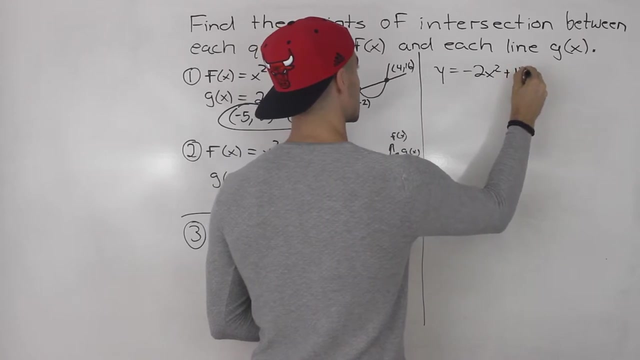 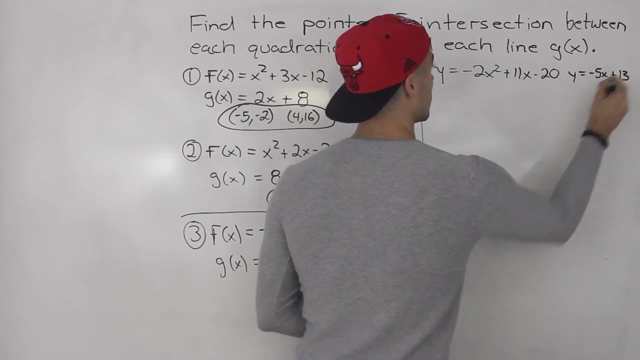 point of intersection. Alright, then, moving on to number three, Let's write out these quadratic, This quadratic in this line: So y equals negative 2x squared plus 11x minus 20.. Then we got y equals negative 5x plus 13.. So, like before, make the y 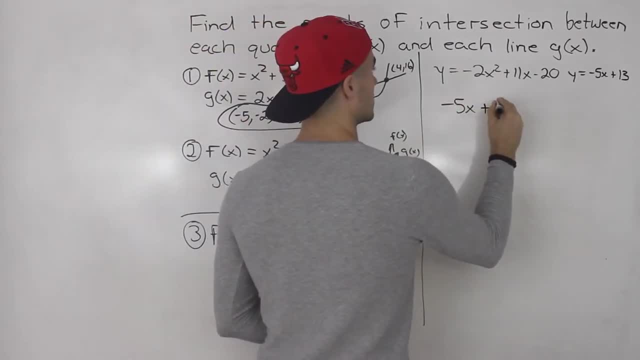 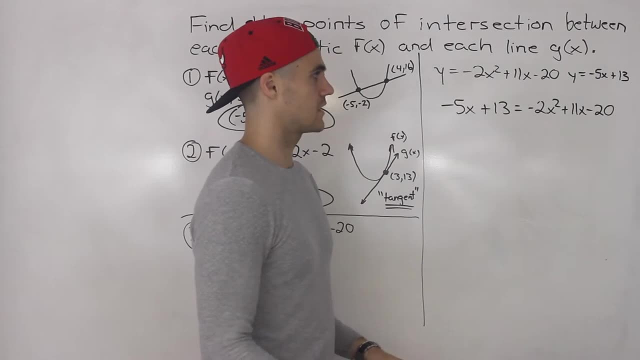 values equal. So negative 5x plus 13.. So negative 5x plus 13 equals negative 2x squared plus 11x minus 20.. And then same thing like before. You want to take one side, bring it over to the other side. 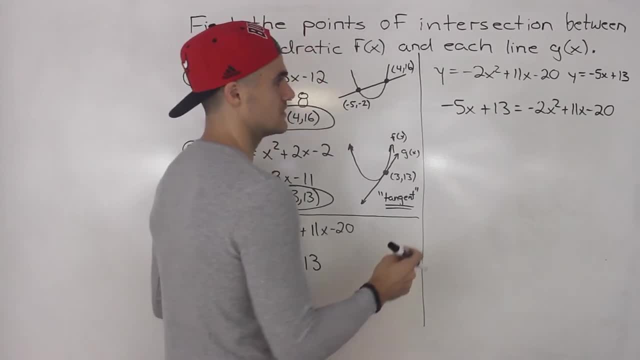 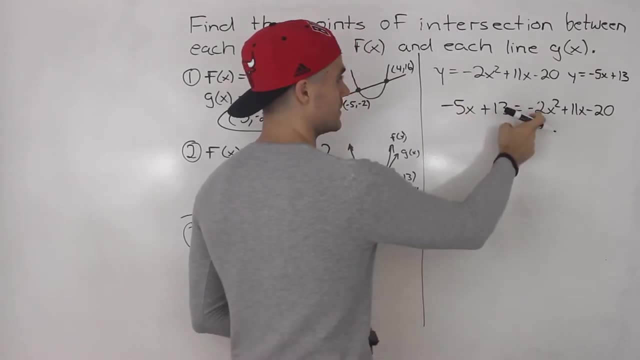 Simplify everything. You'll have a quadratic equation. So in this case I'm gonna take the right side, bring it over to the left side, Just because I usually like that leading coefficient to be positive. So this comes over, becomes positive 2x squared- There's no other x squared here. to simplify it with: And then 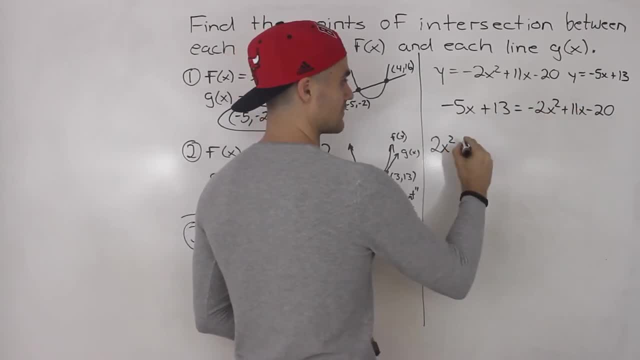 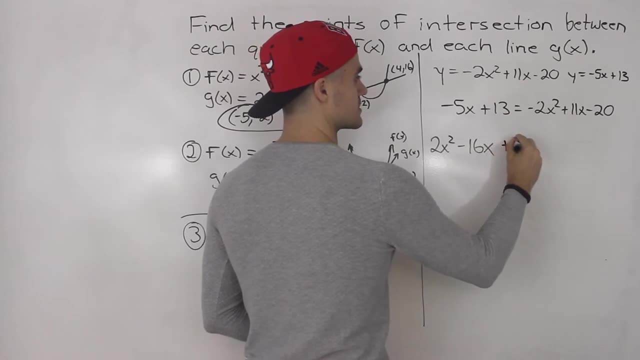 I'm gonna bring this 11x over, So it would be negative 5x minus 11x, which would give us negative 16x, And then 13 plus 20 would give us positive 33.. That's gonna equal zero. 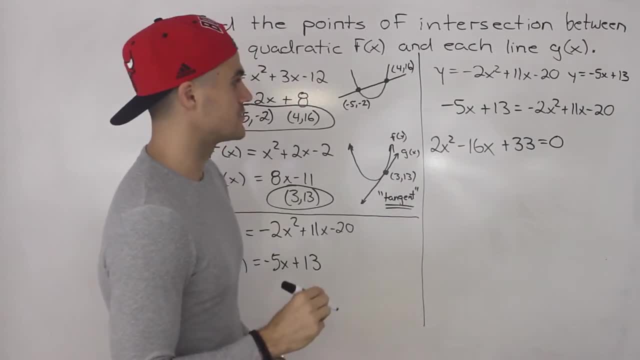 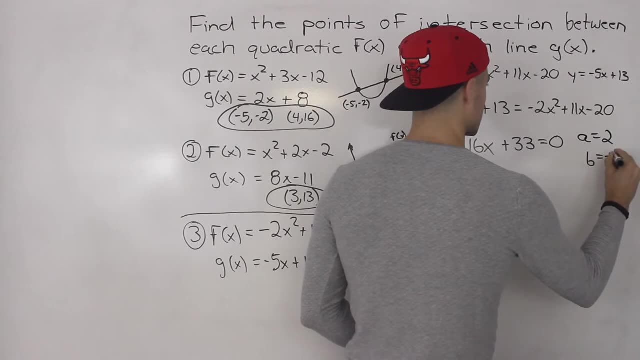 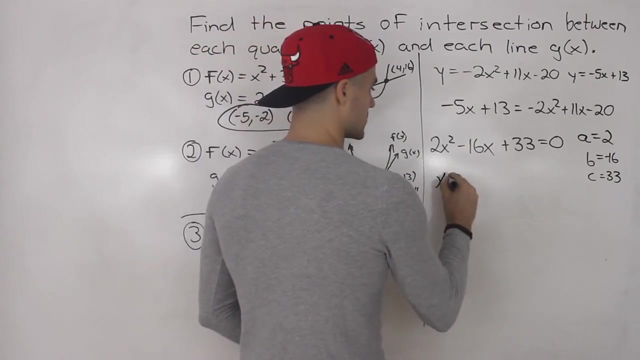 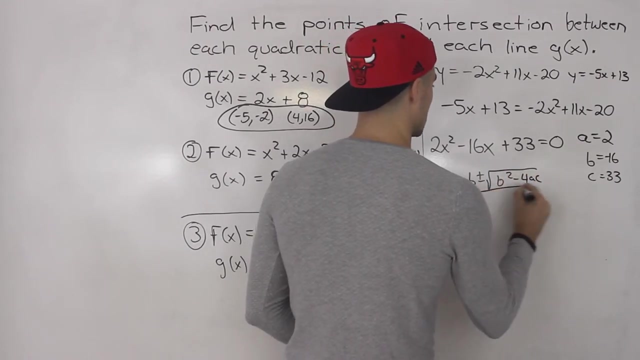 And then from here this actually doesn't factor smoothly. So what you want to do is you want to plug it into the quadratic formula. So we know a is 2, b is negative 16, the c value is positive 33.. So quadratic formula is what Negative b plus or minus b squared minus 4ac, all over 2a. 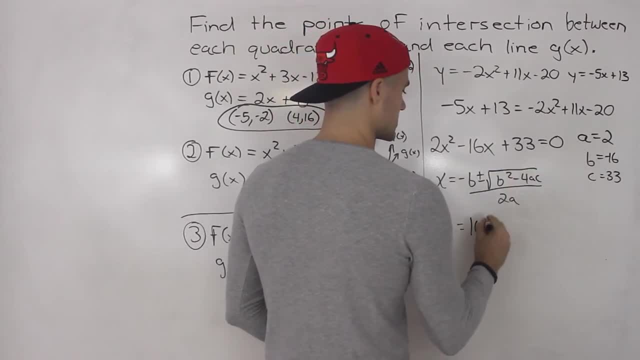 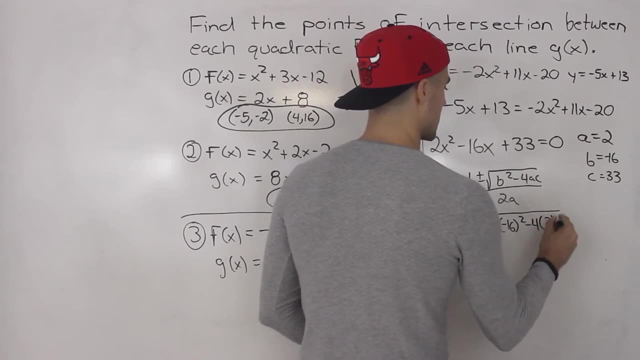 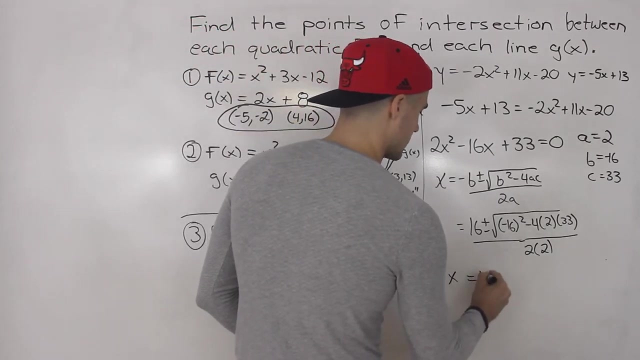 So we'd have negative, negative. so that's positive, 16 plus or minus negative. 16 squared minus, 4 times 2 times 33.. All over 2 times the a value which is 2.. And then what's gonna happen here is: under the square root, you're gonna get: 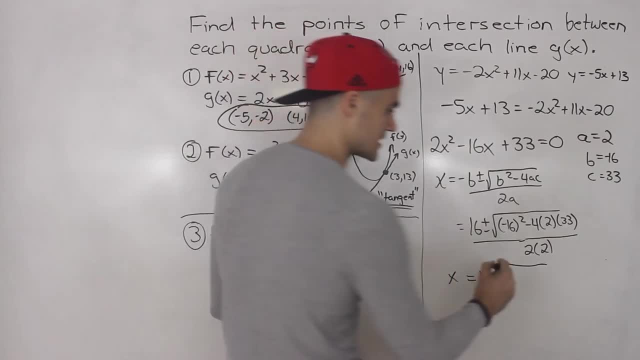 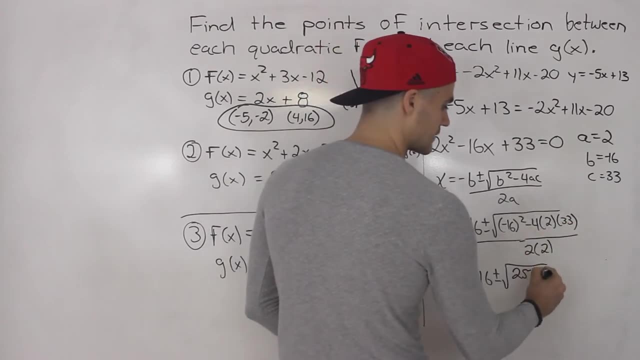 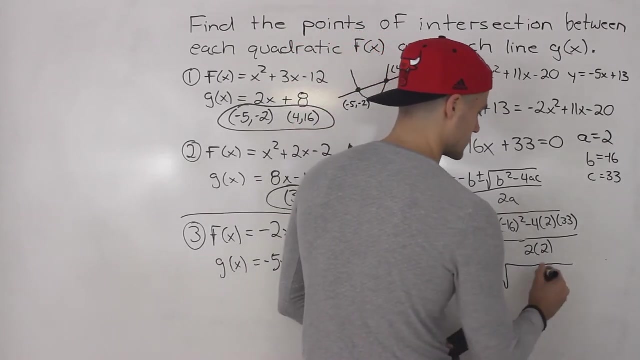 a negative number Because negative 16 squared is 256. And then 4 times 2 times 33, negative 4 times 2 times 33 is negative 264.. And 256 minus 264, that is equal to negative 8.. 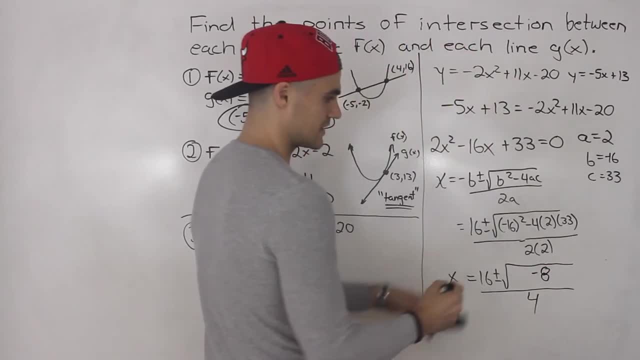 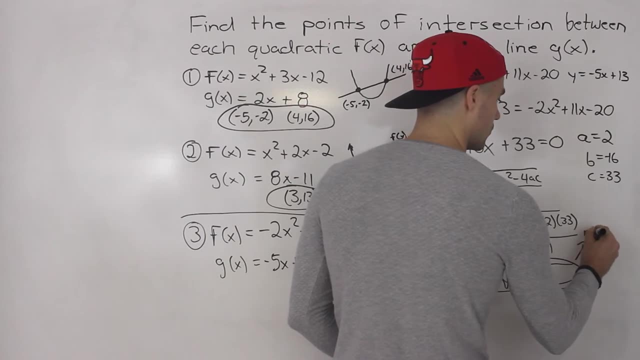 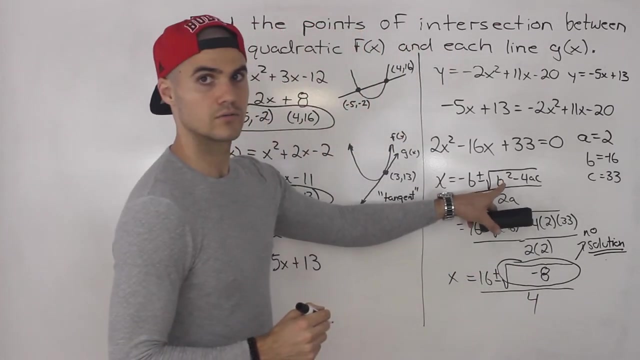 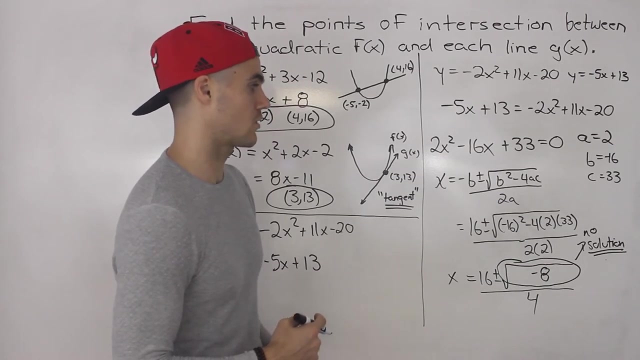 It's gonna be all over 4.. So because we got this here square, rooting a negative, that means that there is no solution to this Right. That's the discriminant. Remember, when the discriminant is negative, there is no solution to the quadratic equation that you are working with. So the answer to number 3 is that there.